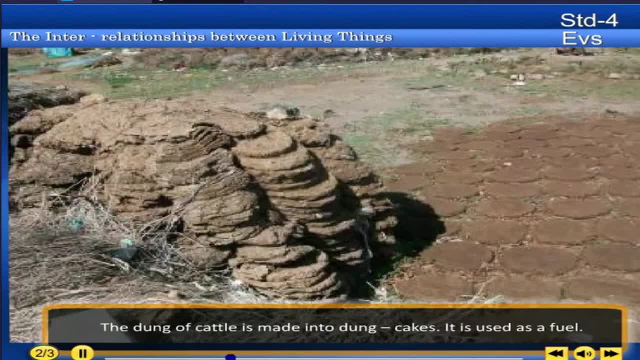 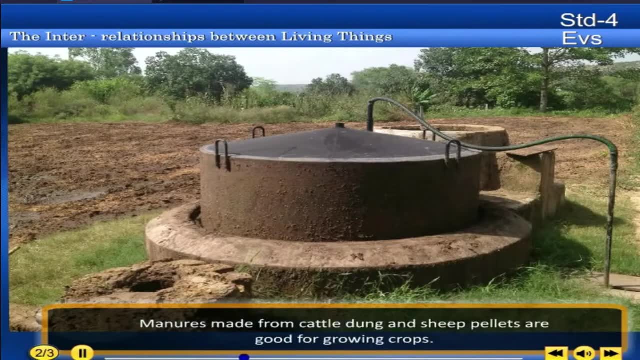 The dung of cattle is made into dung cakes. It is also used as a fuel. A combustible gas called gober gas is also obtained from dung. Manures made from cattle dung and sheep pellets are good for growing crops. We need plants too. 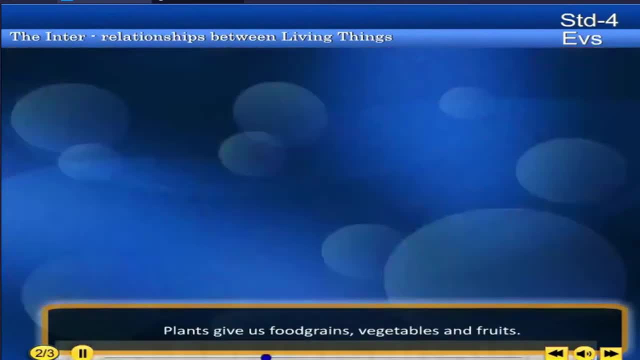 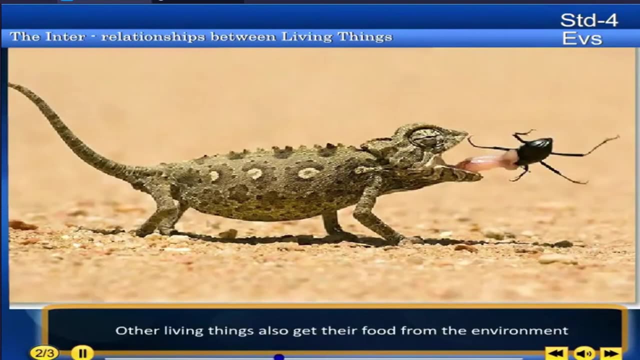 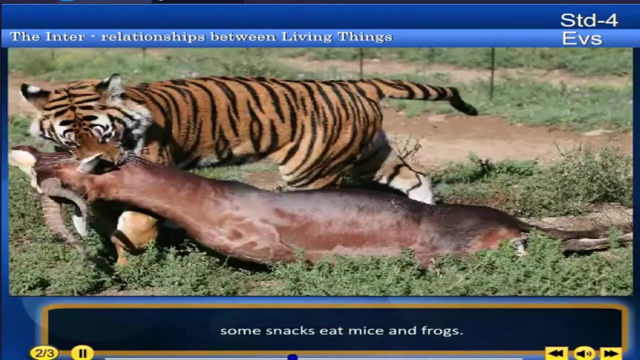 Plants give us food: grains, vegetables and fruits. We also get cotton from plants. Other living things also get their food from the environment. For example, chameleons eat insects, Some snacks eat mice and frogs, Tigers eat deer Goats and sheep eat leaves of tongue. 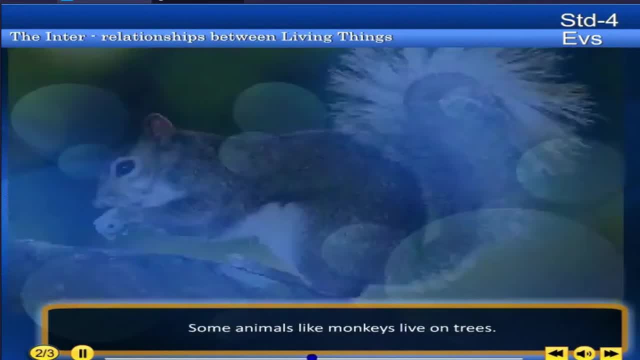 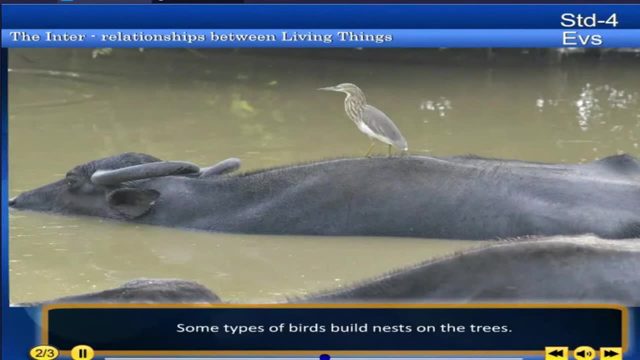 Cattle eat grass. Some animals, like monkeys, live on the trees. Such animals are called arboreal. Some types of birds will nest on the trees. An egret rides on a buffalo's back. When buffalo walks in the grass, the insects fly out of the grass and egrets eat those insects. 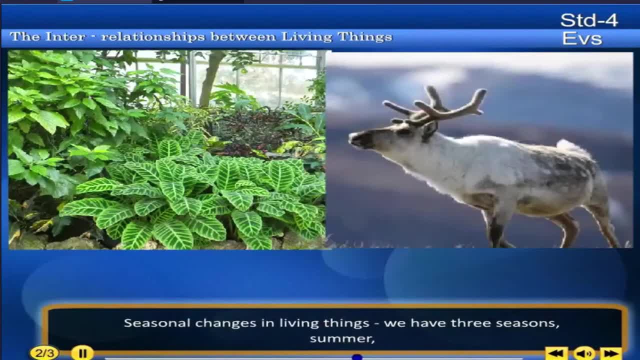 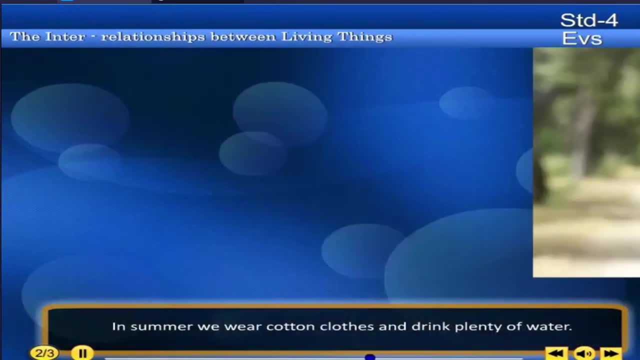 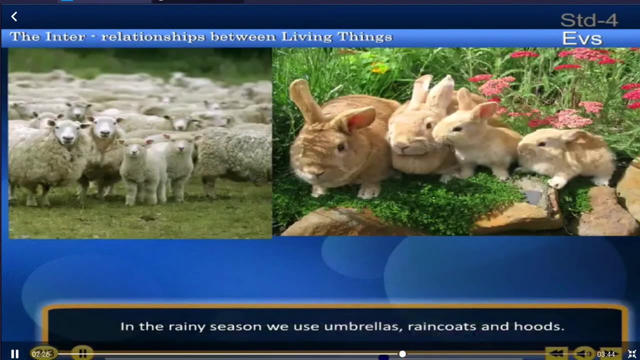 Seasonal changes in living things. We have three seasons: Summer, the rainy season and the winter season. In summer, we wear cotton clothes and drink plenty of water. In the rainy season we use umbrellas, raincoats and hoods. 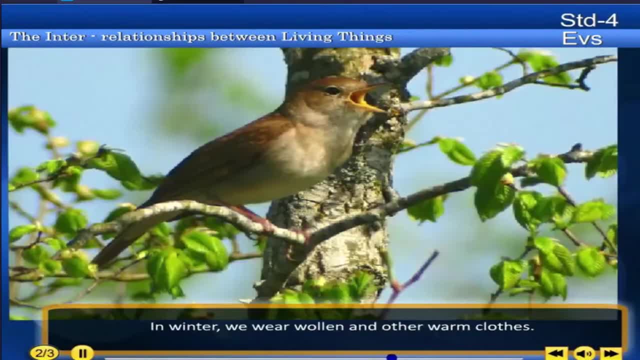 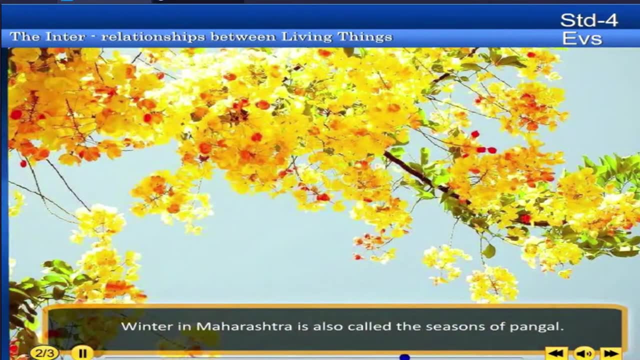 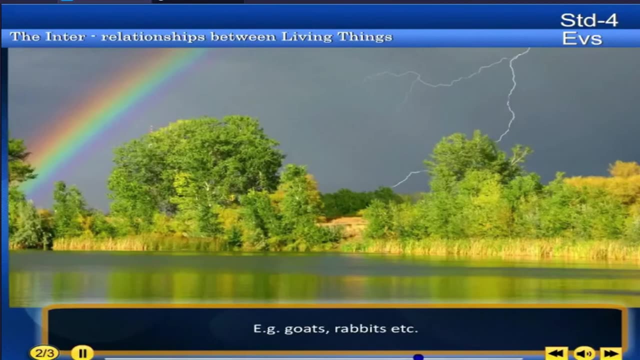 In winter we wear woolen and other warm clothes. Seasons also affect other living things too. Winter in Maharashtra is also called the seasons of pangal. The coats of many furry animals become thicker in winter, For example goats, rabbits, etc. 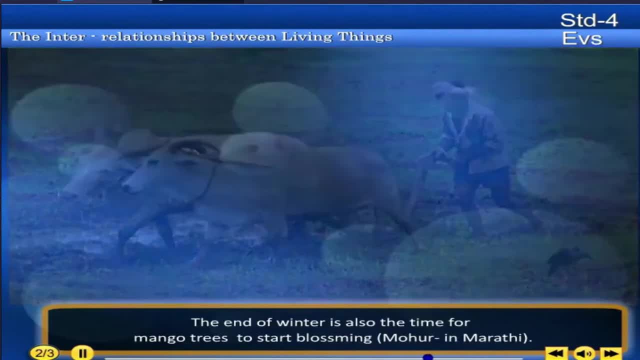 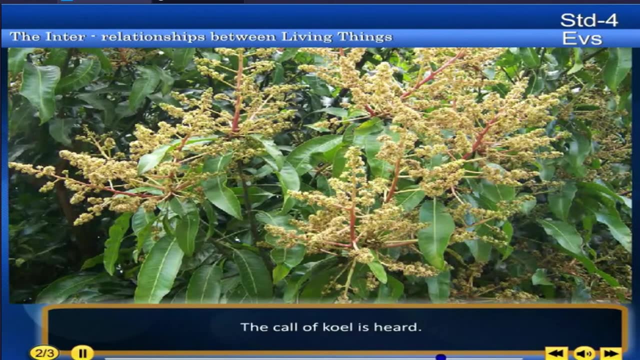 The end of winter is also the time for mango trees to start blossoming. Mohar in Bharati. In summer, many trees get new leaves. The call of koel is heard. In summer, the market is full of mango trees. In summer, the market is full of mango trees. 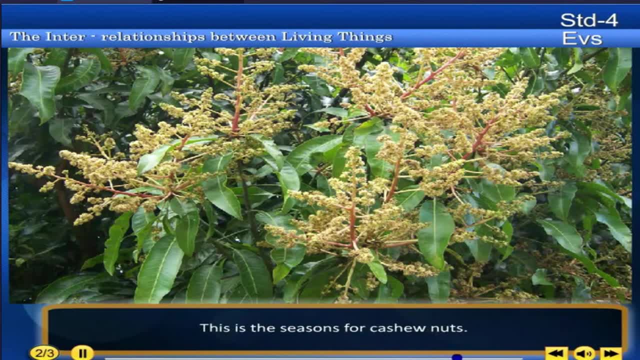 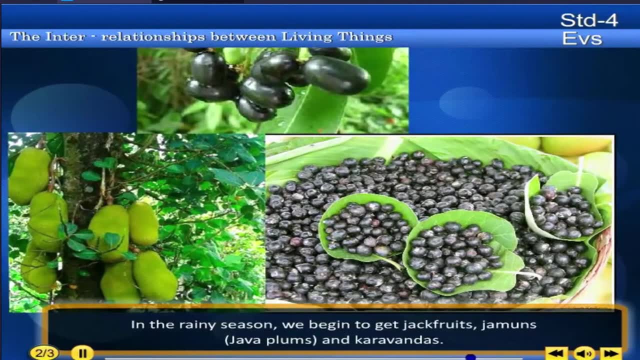 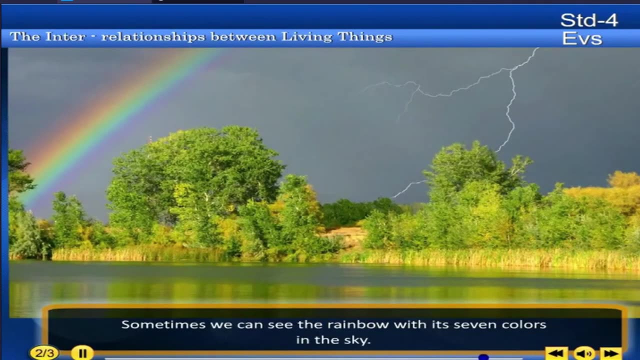 Mangoes and watermelons. This is the season for cashew nuts. In the rainy season we begin to get jackfruits, jamuns, java plums and karmandas. Sometimes we can see the rainbow with its seven colors in the sky.